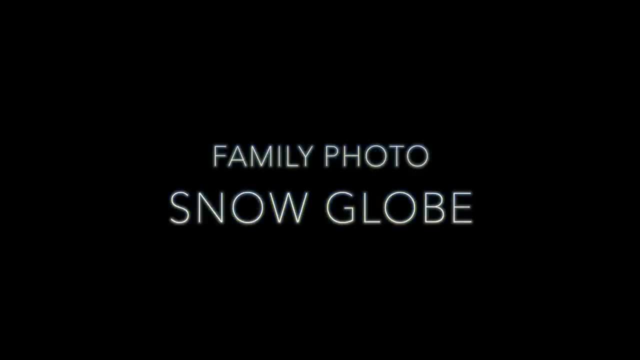 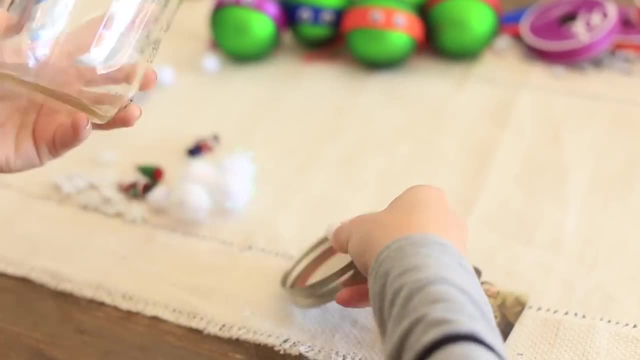 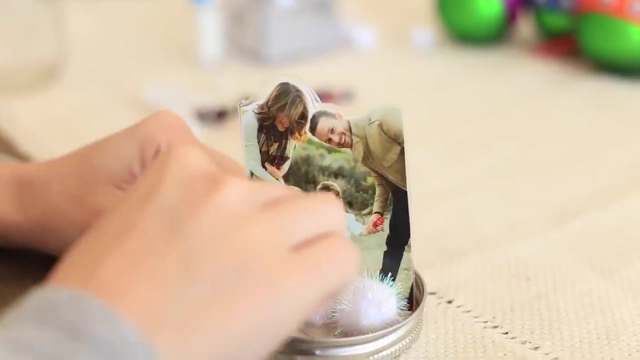 this might be a hit. Next, we're making a family photo- snow globe. Now you can do this with any photos that you want, You just have to laminate it. I took a family photo and then used a mason jar, a hot glue gun. the picture really nice and tightly. as much hot glue gun as you can get in. 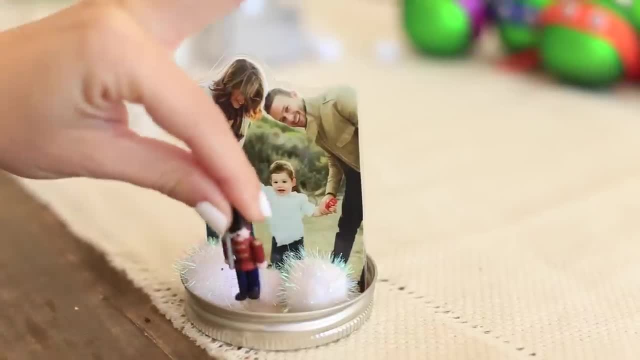 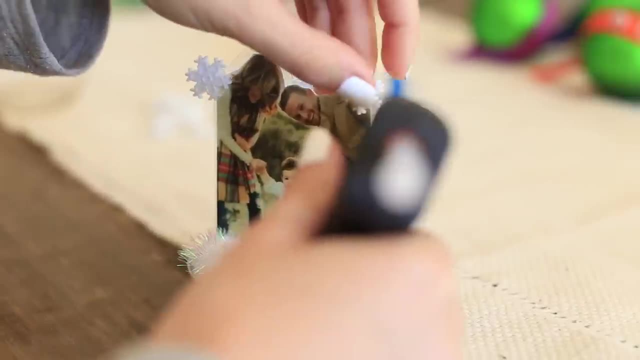 there. And then I surrounded the area that had the glue with, um, what I thought looked like snow and a little nutcracker, and just kind of decorated it a little bit so that you don't see the glue. And then I also glued on top of the picture, um, some snowflakes. 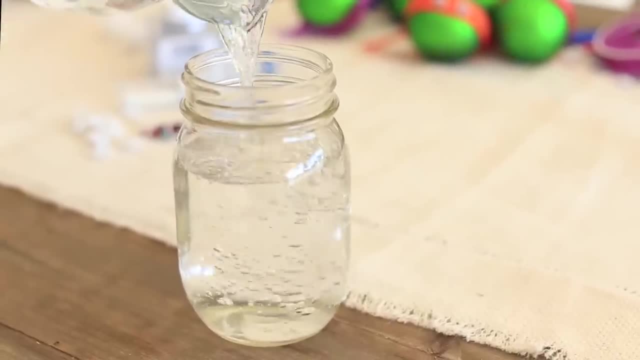 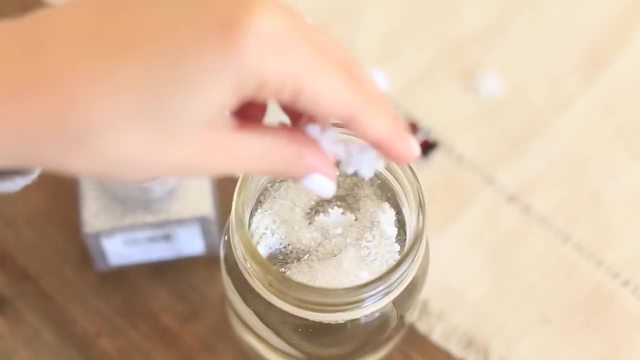 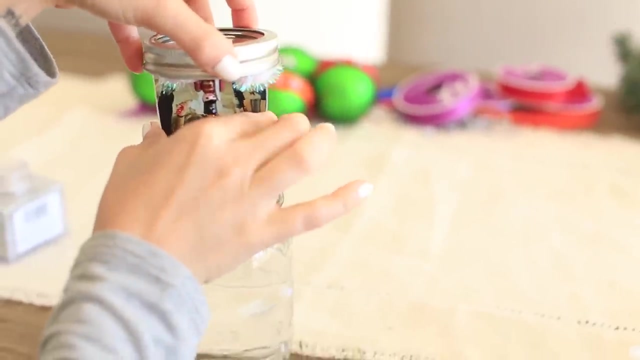 and decorated it. I'm adding water to the mason jar and then glycerin, So you're going to need about, I would say, one tablespoon approximately of glycerin. I'm adding some glitter snowflakes and then I'm going to put the top, very gently, inside the snow globe after it's had a chance to. 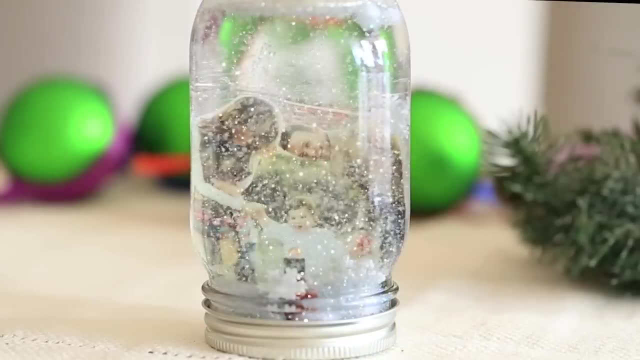 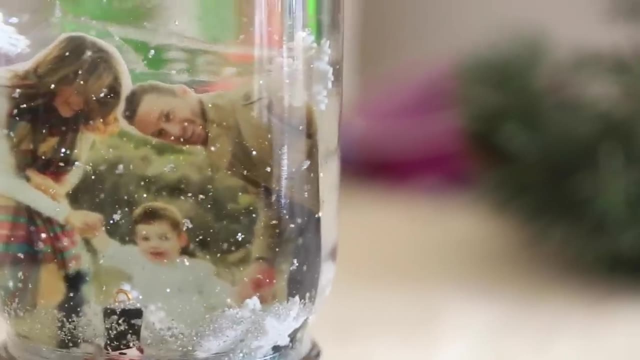 dry and shake it up And you have a really wonderful gift. I think that this is a fun gift for grandma, maybe with the grandchildren in it, or a gift for anyone really who would like that and appreciate it. I honestly think anybody would appreciate this hot chocolate ornament because it. 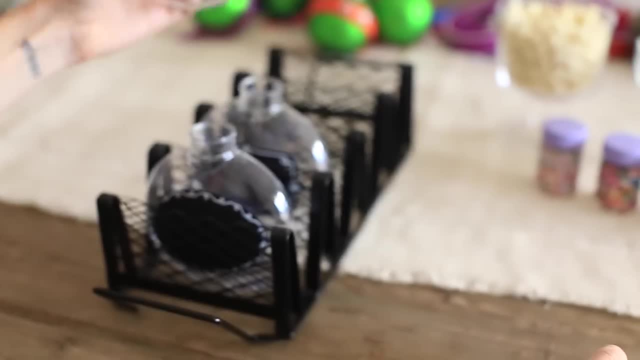 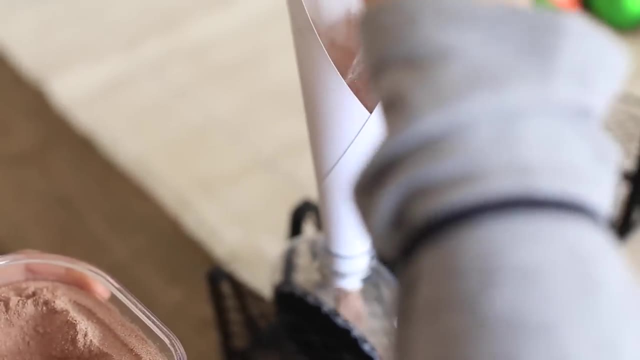 is so fun. So I got these little ornaments that have just like a little chalkboard on the front at Michael's. I'm using this little taco container that Byron has for cooking and I created a little funnel and I'm adding some hot chocolate to it And then I'm going to add a little bit of 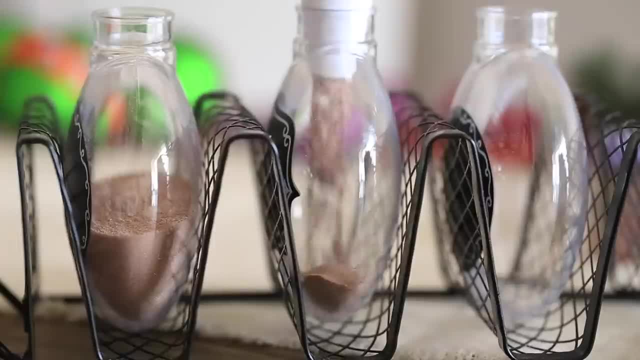 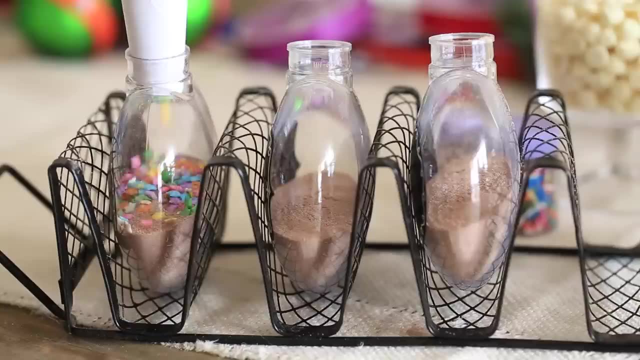 hot chocolate mix into each of the ornaments. Now you want to read the instructions um to add the perfect amount of mix and then let them know how much water they're going to need to add to this. Then I'm going to layer it on top with some sprinkles- different sprinkles for each one. 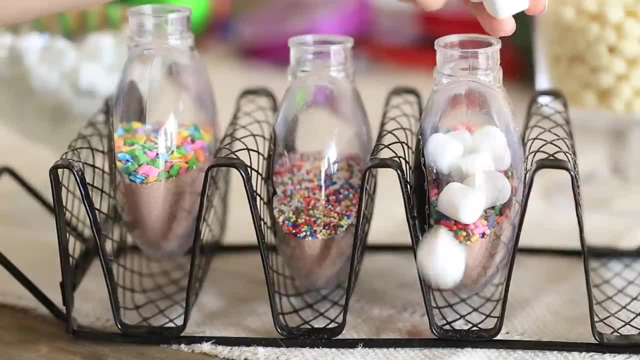 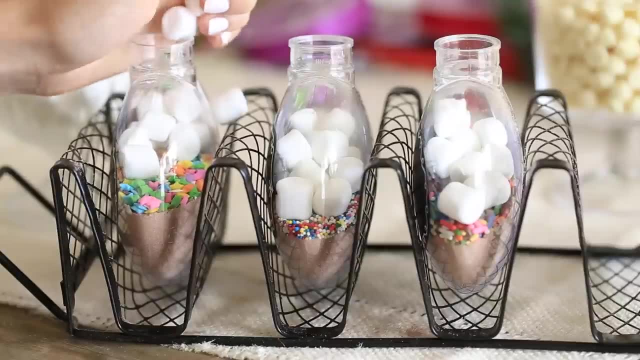 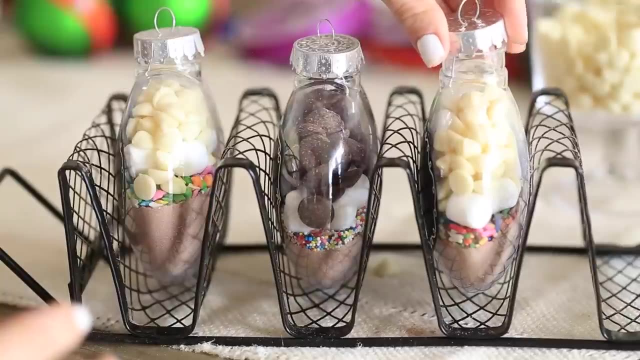 Then we're going to add some marshmallows and you can pretty much add whatever you want, but it's basically just making a ready to go hot chocolate and you just add water. So I thought that this was really fun. This is a fun and easy gift that can be made by kids or adults for kids or adults for. 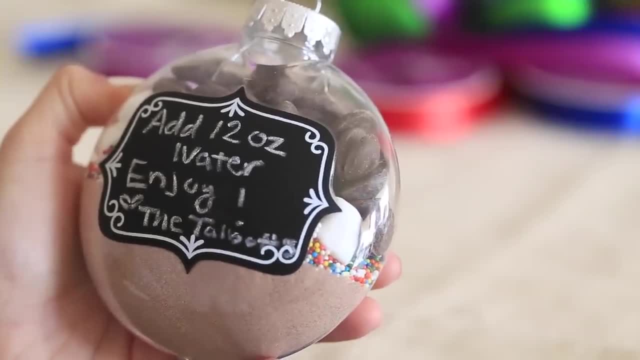 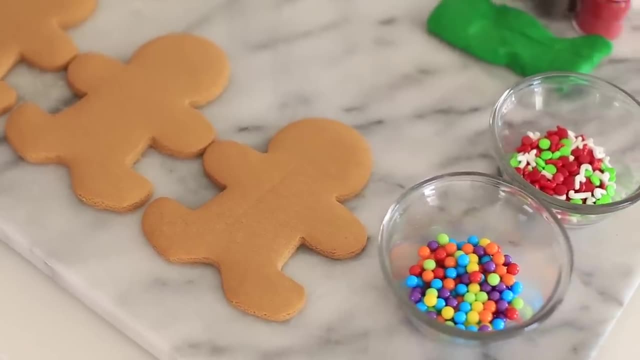 parties, um, or teachers. All you have to do is tell them how much water they need to add and who it's from. Next, we're doing a fun gingerbread making bar with kids. You can do this for Christmas parties or events or just some fun time with your kids. You can either make the cookies